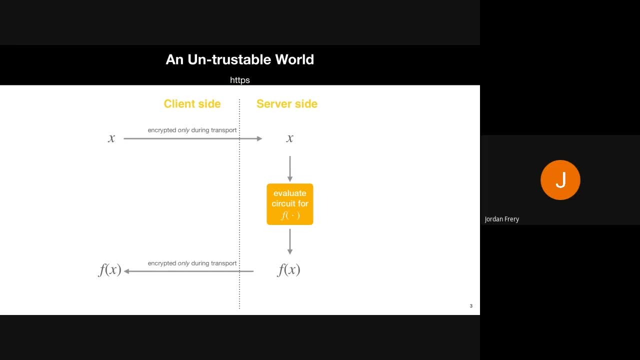 a complicated task. you often don't do this locally, so you just send the mail to the server. You've got to send the whole clear text to the server And the server executes the algorithm to detect whether it's spam and it sends you back the prediction or the probability. 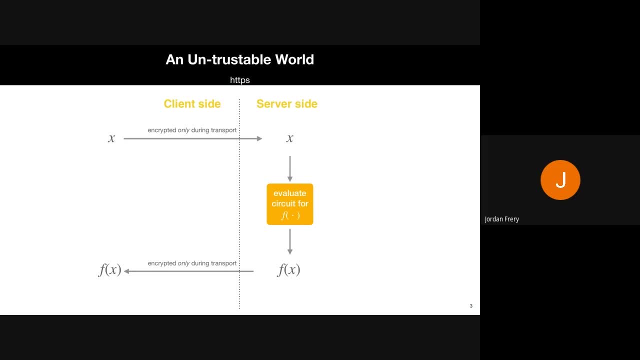 of the mail to be a spam or not. So of course there is a bit of a problem here, since there is some kind of trust that is implied because the server not only has access to the spam your mail but also has access to the prediction, which basically gives a lot of information. 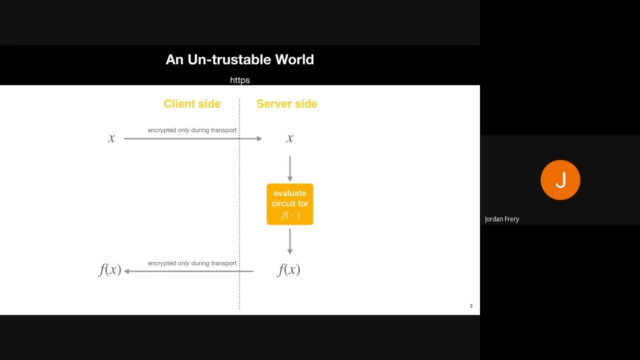 about the client. So what is FHE? FHE aims at providing a privacy for the user. So what happens is that- let's take the spam detection example again- You take the mail, you would encrypt the mail locally at the client machine and you would send this encrypted data point to the server. 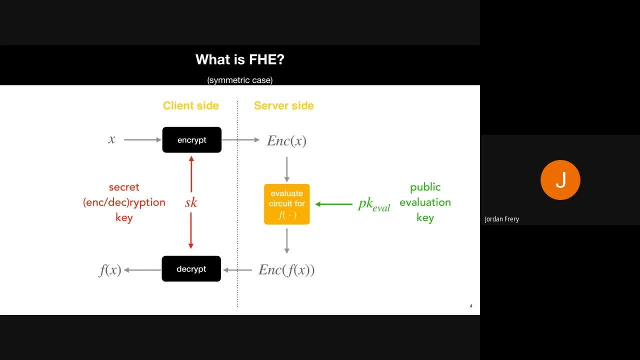 And the server, thanks to fully homomorphic encryption, would be able to execute the same function as it would have done on the clear data and send you back the encrypted results. Of course, it applies the function of the encrypted data, The result of this function. 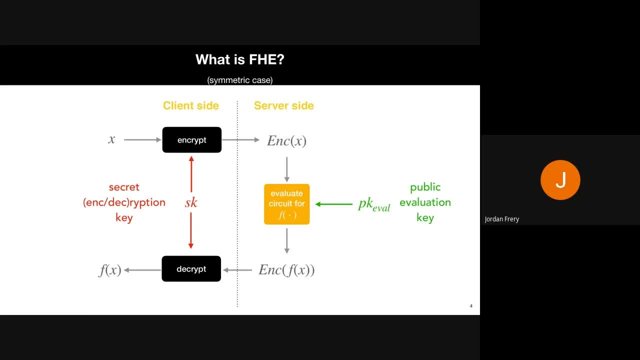 is also encrypted, And only the client which has access to the private key which it used to encrypt the data can decrypt the results of the function that has been executed on the server. So let's dig a bit more into FHE. Here you are represented: X and Y, which can be two. 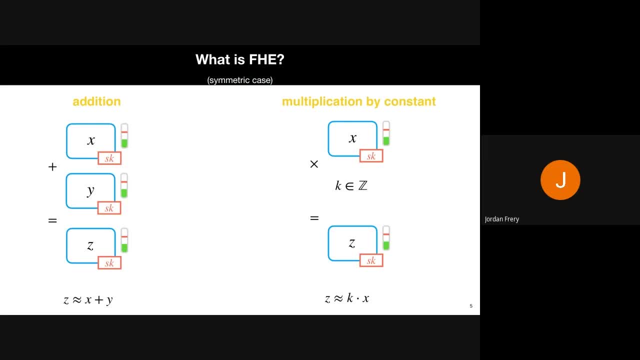 data that have been encrypted. So let's take a look at FHE. Here you are represented X and Y, which can be two data that have been encrypted. We have a specific private key In FHE to maintain the security. you have some noise in what's called the cipher text. 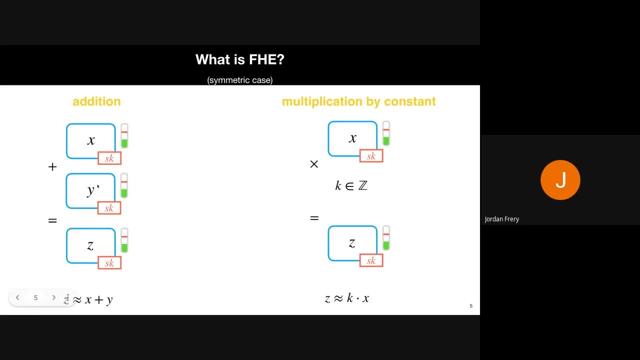 So the encrypted X and the encrypted Y, You have some noise which here is represented by the green level here. So when you add them together, so two cipher texts together, you encrypt these codes. So increase very slightly the noise. so if you would do a very long sum it would increase more. but 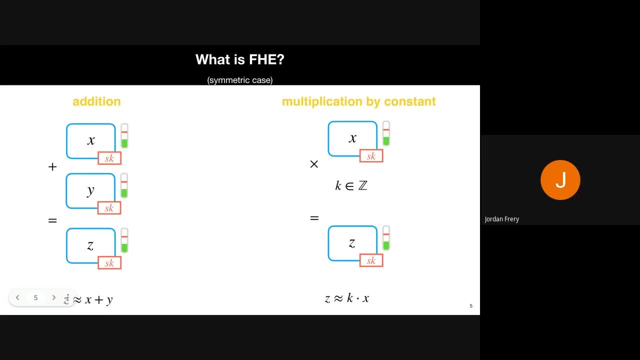 so this is how uh having operation fhe works. so you would having arithmetic operation between two ciphertexts would uh um, increase the a bit the noise, but that's not too bad here. for the addition with the multiplication, same thing if you multiply a ciphertext with a constant, the. 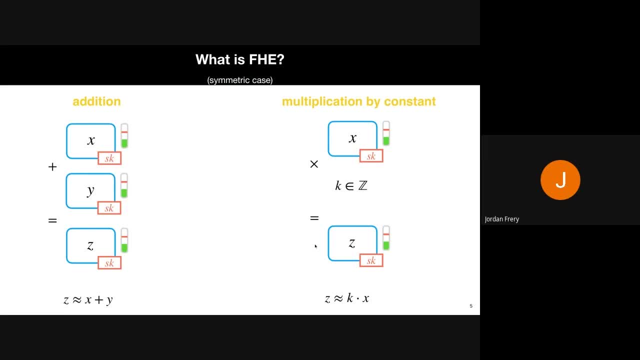 noise remains kind of stable. so what i mean by stable is that once the noise reached this red level here, what happens is that, oops, what happens is that, um, then the noise is basically um overwriting, like the, the actual data, that is, that's been stored in the, in the, in the ciphertext. 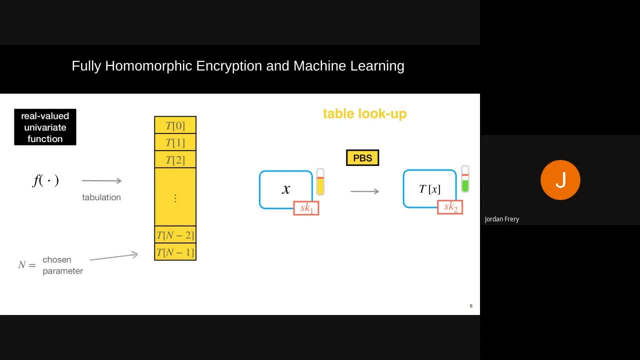 so when you do a lot of computations you will arrive to a point where the noise is quite high. so in fully homomorphic encryption there is something called a programmable bootstrapping, which you call here pbs. in at our level, at the machine learning level, this programmable 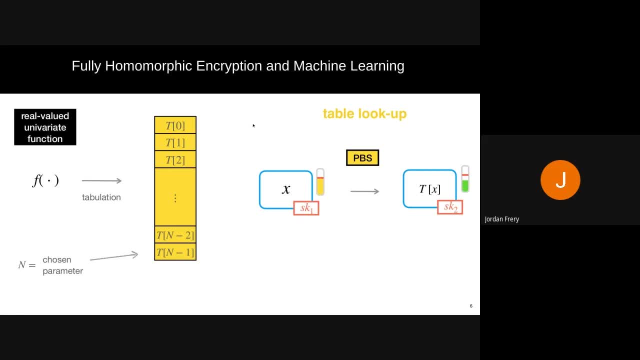 bootstrapping can be seen as a simple table lookup. so essentially just mapping, just any variant, mapping any varied function from an integer to another integer, right, and this is quite interesting because this table lookup allows us to have some kind of non-linearity in the fhe circuit, but also when you apply a pbs. 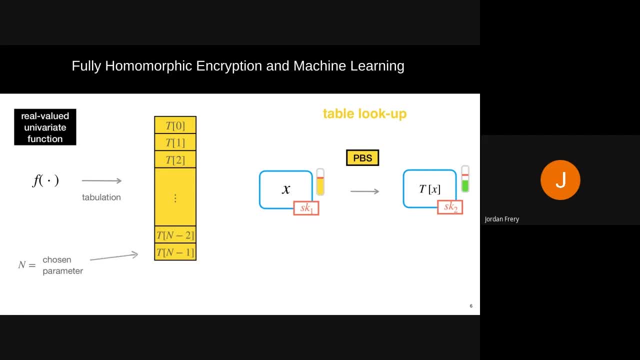 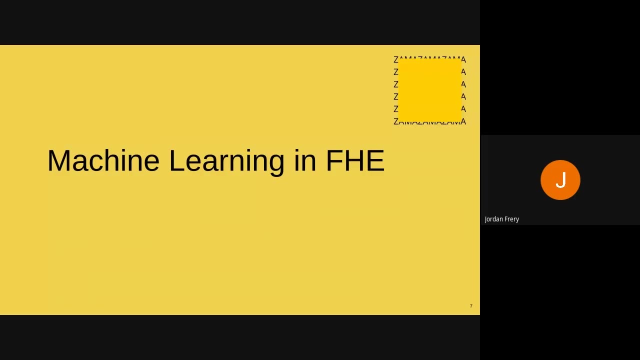 it decreases the noise. so you can keep working with this, this ciphertext that comes right after the pbs. so this is why machine learning becomes very interesting in this case, because you could have very long circuits and always play around these pbss to decrease the noise and keep going with the 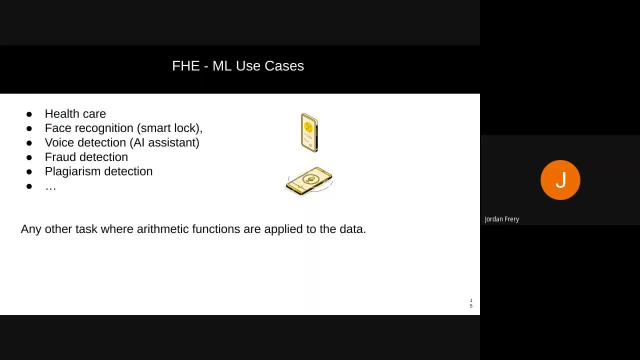 computations. so let's tackle a bit more machine learning use cases here. so, of course, the first one to mind is based on healthcare, where machine learning is a bit stuck today because of abuse reasons of data being very sensible to share and compromises some privacy from the users. 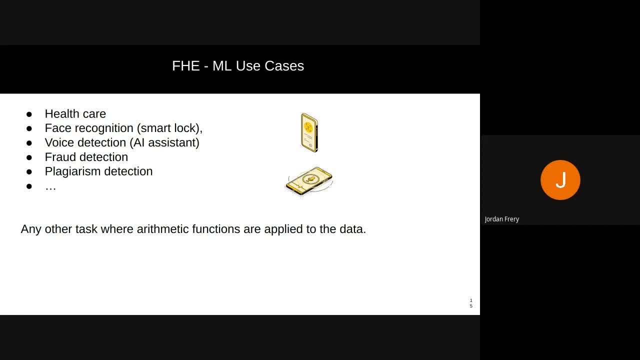 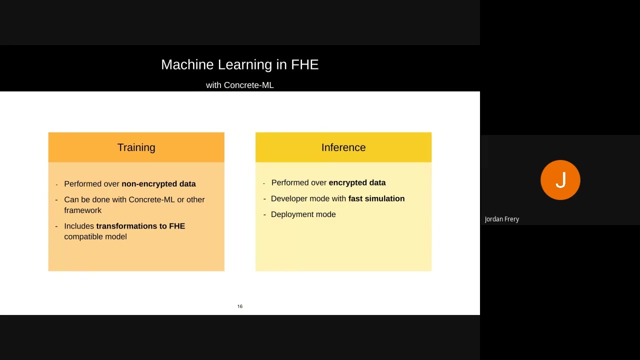 of course there are a lot of different applications that can be done, like face recognition, voice detection, for detection, basically only arithmetic functions. uh, can- that represents machine learning models- can be done in fhe. so machine learning. currently, with the fully homomorphic encryption um that we have now we are performing the training of the machine learning model on 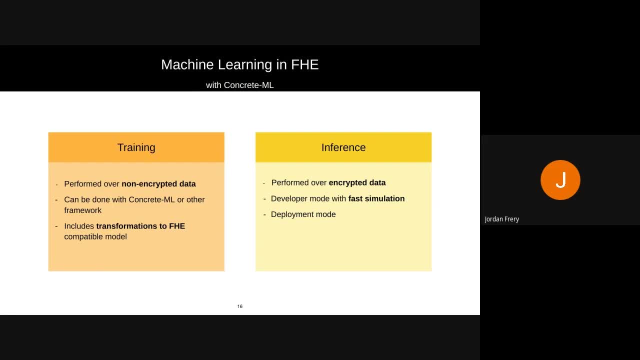 non-encrypted data. it can be done with the open source library i'm going to present right after the demo um, but it can be done with anything uh you'd like, and the library is supposed to convert any machine learning model to its fhe equivalent, and the the pros of concrete ml for now is to allow the inference. 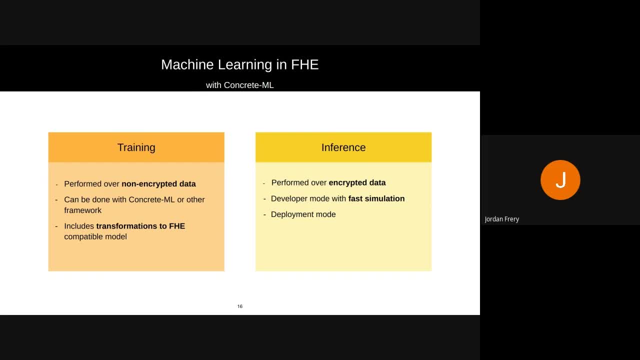 um, pass this to concrete ml and you would get an fhe circuit which is with the, the crypto parameters, to encrypt the data. so you would have to create a private key as a client, you would have to uh, the secret key as well, and um, and then you could deploy the fhe circuit in a untrusted 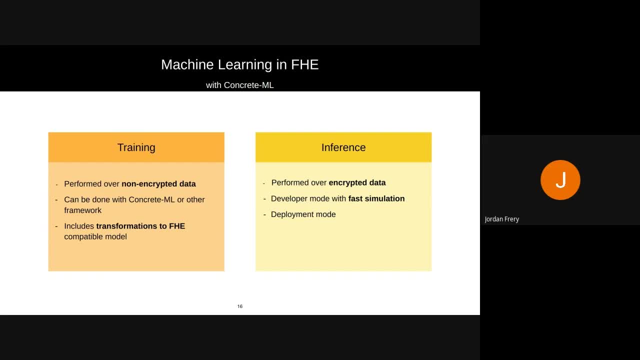 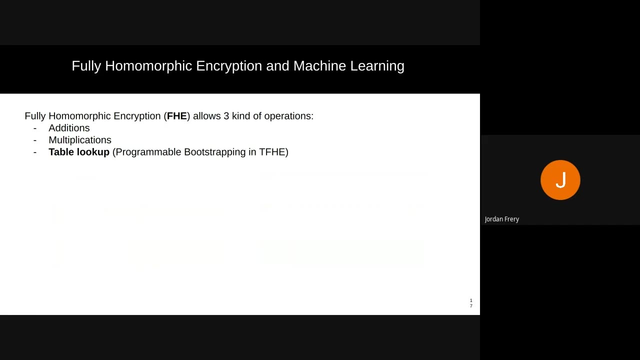 server which would run the inference of encrypted data. so we provide also in this library the, the fast simulation and the deployment mode. uh, i might come back to this later. so fully homomorphic encryption, uh, as just said, basically imply three kind of operations, so additions, multiplications and this programmable bootstrapping which for us is going to be a table. 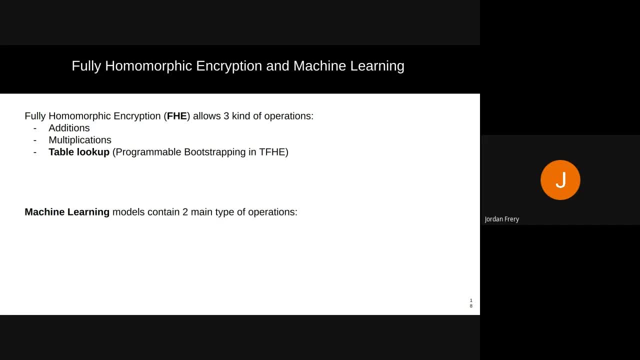 lookup a very simple table lookup and in machine learning what you would get is matrix multiplications, which represents, like more than 90 percent of all the operations you actually do um in in machine learning models. so multiplication and additions, those are pretty fine, uh, to do in. 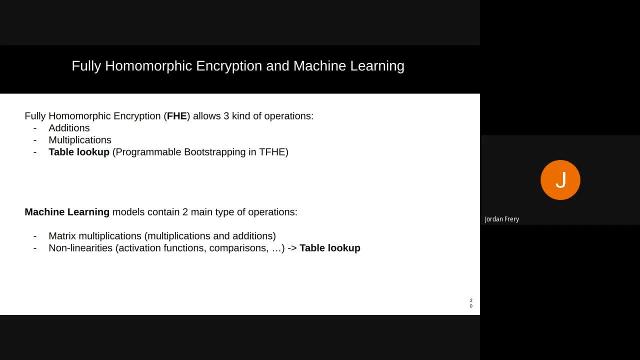 in a morphic encryption. and the second part is non-linearities. so in neural nets, for example, you want to break the linearity by adding some activation function, non-linear automation functions- uh, you could also have, as we will see, in trees. you have some comparisons between values. uh, that breaks the linearity and this is going to be represented. 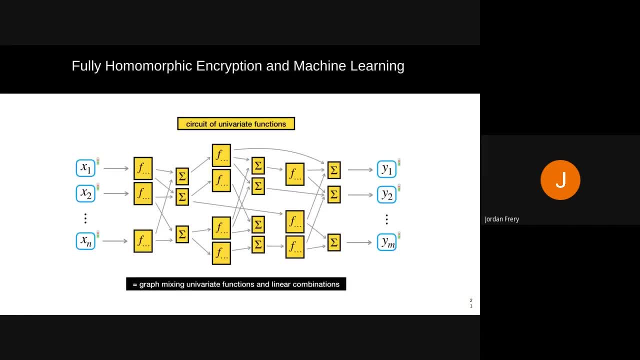 using a table lookup. so overall fully homomorphic encryption and machine learning can be matched by having a more telegram library, two kind of uh main operations, uh so you have the ciphertext, uh so encoded and could uh encrypted inputs that comes in the machine learning model that can do whatever kind of computation. 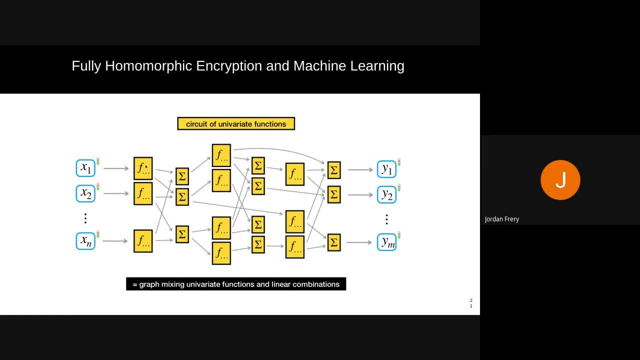 it needs to be done. so here the function represents the pbs's, so those could be non-linear activation and you want in fhe to represent that the. then, with a table lookup, the sum would be just, you know, matrix multiplication, and, and then you can, thanks to the 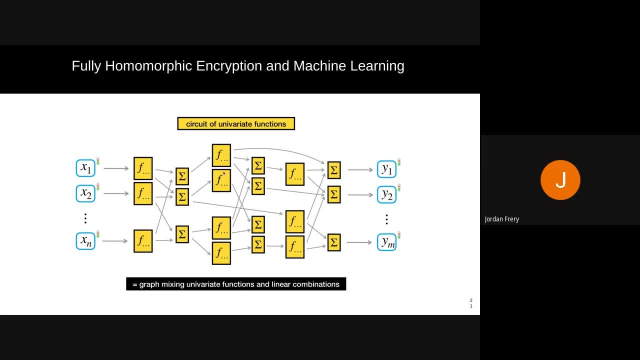 pbs's, so the functions. here you would be able to go very deep without actually destroying the ciphertext because of this noise increasing, since you can actually use the bootstrapping to decrease the noise step by step. in neural nets these pbs's happen every, at every level, often at every level. so 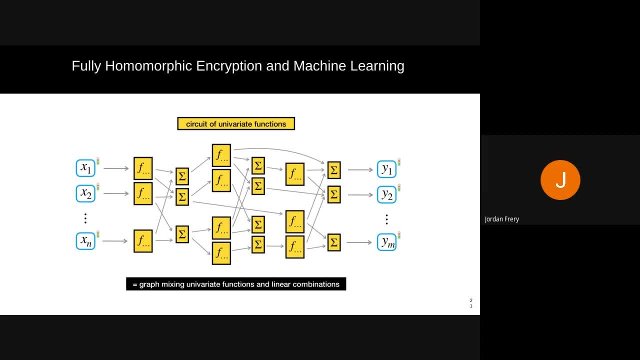 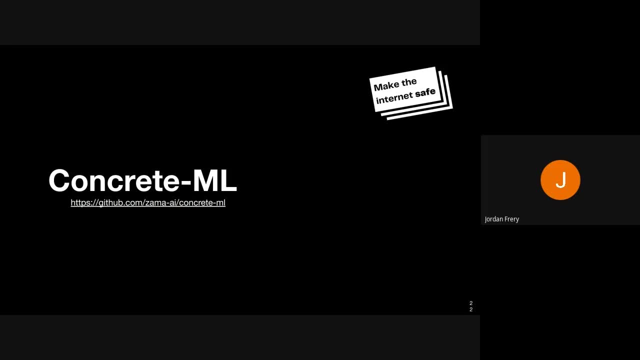 after matrix multiplications, convolutions and then things like that- great. so now um let's uh have a look at concrete ml so it's available on github publicly. we are we are trying to release every every three months um updates uh, as we are working with uh the research uh teams um that work on. 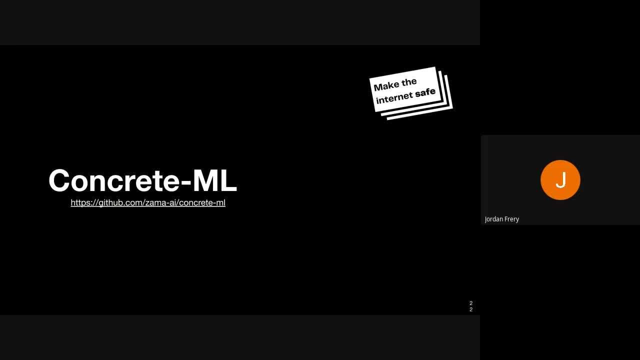 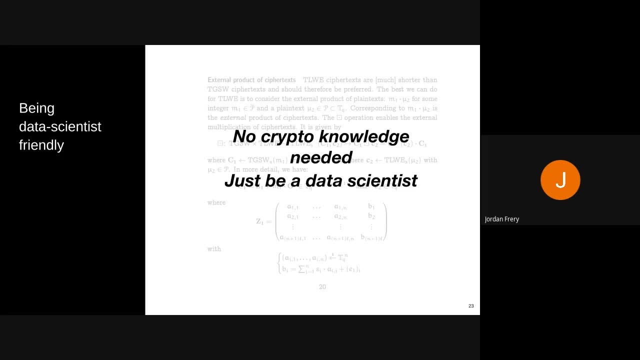 fully homomorphic encryption. uh. we bring a lot of different um improvements every, every every three months, so you can check it out. and github. this library has been designed so that um people that with absolutely no crypto knowledge, uh- could actually use it, so we're going to go ahead and 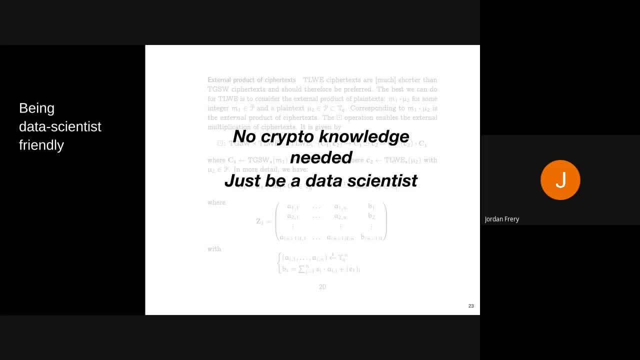 the only thing that uh will be needed to know is, um, that you have to create uh keys and, and, but basically training the model and deploying would be very simple. here we try to be as close as possible as what data scientists and machine learning practitioner are used to to have. 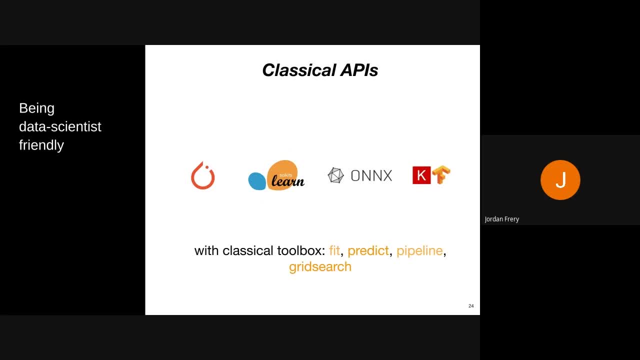 so in those there is like we support torch and and tensor flow, but also all the models, most of the models that are available in a circuit, learn and onnx we are. it's a representation of machine learning models using a kind of graph abstraction, and it turns out that most of the machine learning 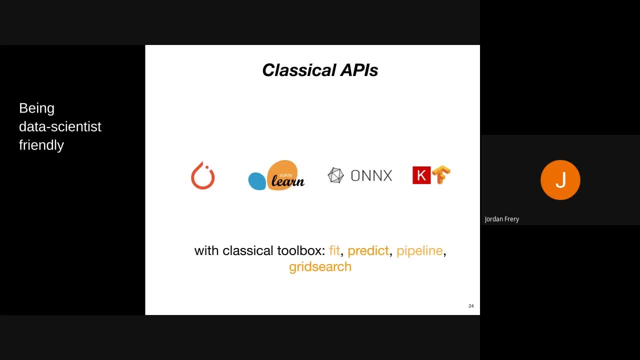 framework can be converted, model can be converted to onnx, which is the main entry point to concrete ml. so of course we have the all the popular api that you can have in python when you work in machine learning with the feet, training your model, predictor, other some data and you have. you have some pipeline and grid search also supports. yeah, 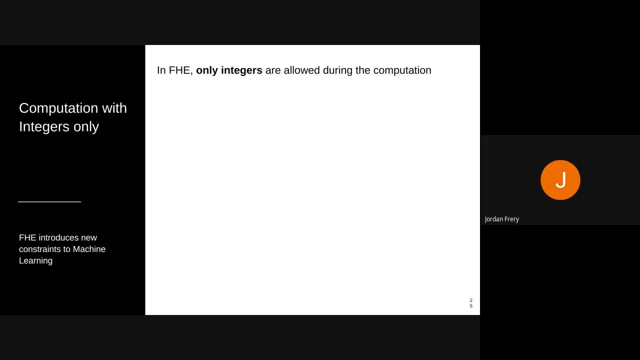 so. so now let's dig in how we actually change the machine learning model to make it fhe friendly. so in fhe, at least currently, we can only work with integers, so computation have to be done with integers only, and to do this quantization. we use quantization, which is an approach that 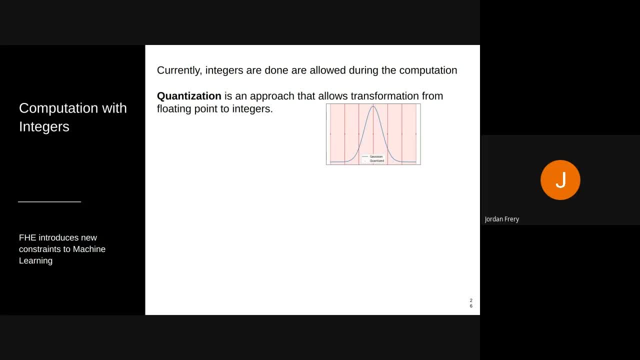 allows transforming floating points, floating points to integers. so if you take a, a distribution like the question distribution, you just cut the distribution of the full range, or you can actually choose different quantile if you want and you define an, a precision which would be like, for example, eight bits on or four bits. 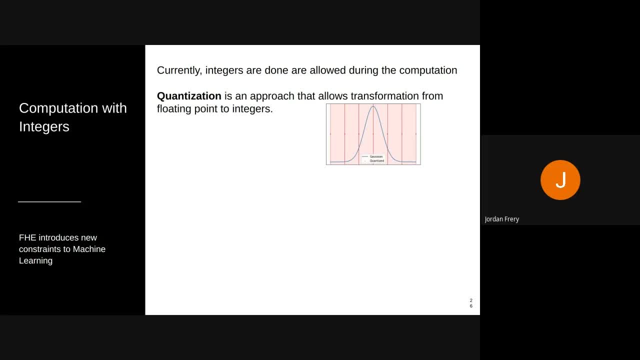 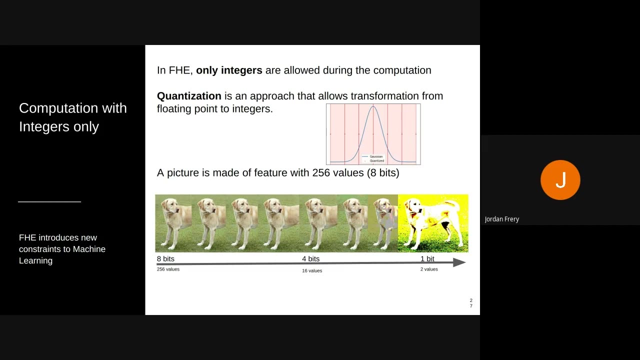 and you cut to your space into the number of available precision. it doesn't have to be x elements. so, quantity of pixels. there's a quantity of pixels, uh, a more visually example. more visual example would be: uh, with pictures, every pixel in the picture is represented with 8 bits, so 256 values. if you would quantize the, the picture, you'd see. 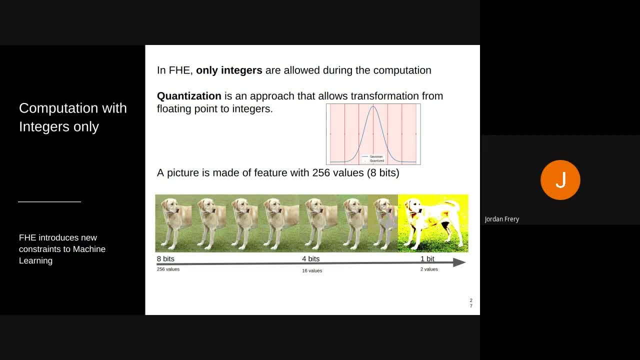 that you would lose some information along the way until you reach a single bit here which allows to have- uh, because there are picture close to have some kind of similarity. but if you would feed the right picture to a machine learning model while it has learned over the first picture, the eight bits one, then you would get some. 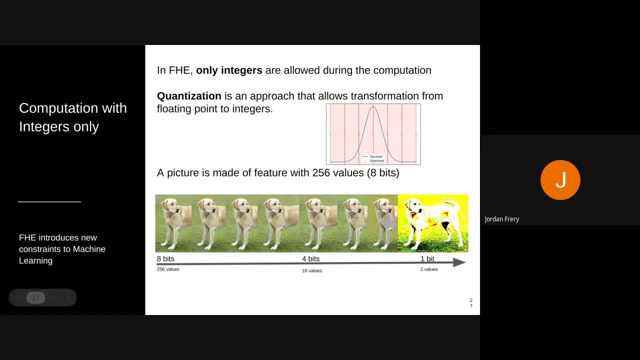 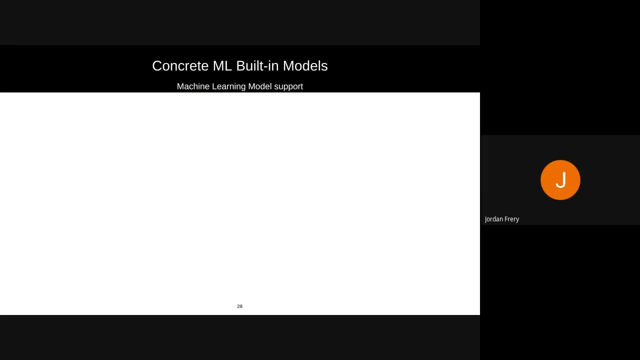 kind of loss in the accuracy. so let's look at what's available in uh in concrete ml and what kind of machine learning model we support here. so the first kind of model are tree based model, so decision trees, random forest and and attributes, which is a gradient boosting algorithm. 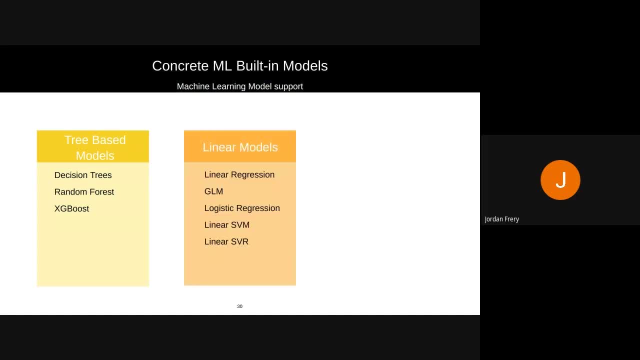 pretty popular in machine learning. then we have linear models, uh. so basically linear regression, a generalized linear models, uh, logistic regression, svms and and others and finally others that appear here: svm, elastic net, lasso, reach, and then finally we enter the world of neural networks. we have built-in neural networks such that user can 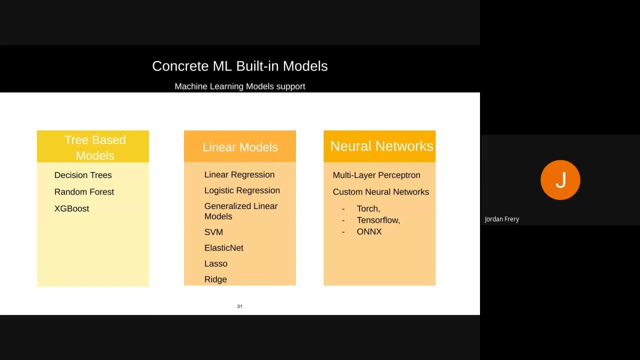 actually train their neural nets, and the neural net is going to be converted to fh instantly. or we can also design the neural network using torch tensorflow onnx if you will, and once the neural net is learned you can basically push that to concrete ml which will do the conversion to the fh equivalent. so let's take a look at tree based model here. 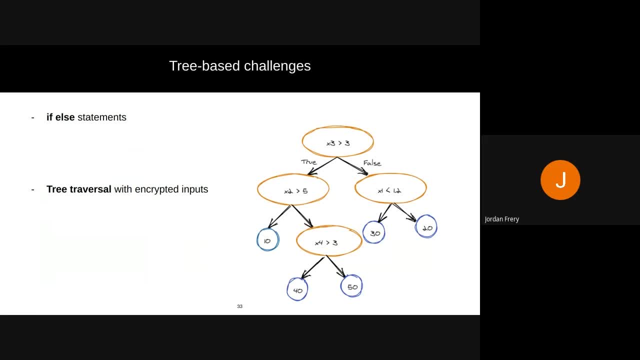 the tree-based model have a challenge which comes from the fact that they are built with if health statements, so in a tree traversal with an output of Meslisted node, with the primary region of n testament making the horizontal line, and if we have meetings of these��서. 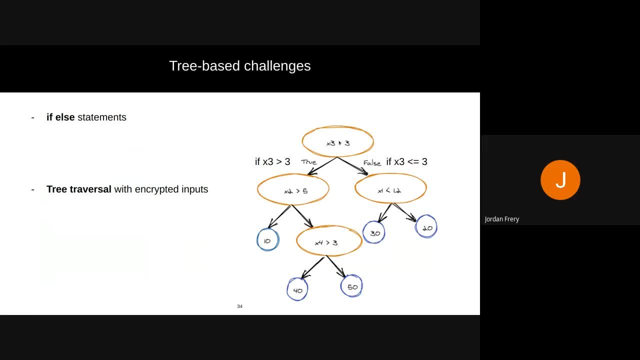 such as k-2n. we have multi-"xbrual decrease가량RicrmR cloth addrp shows stock timeűof your eigen Repression. so on that gradient extension, there's noroеко salad. align to a Felipe. so this node input, you would have to do a comparison with encrypted input. you would have to do comparison between, uh, the, for example here the x3, which would be encrypted, and a clear value which would be in the clear um with this, this kind thing, but comparison. 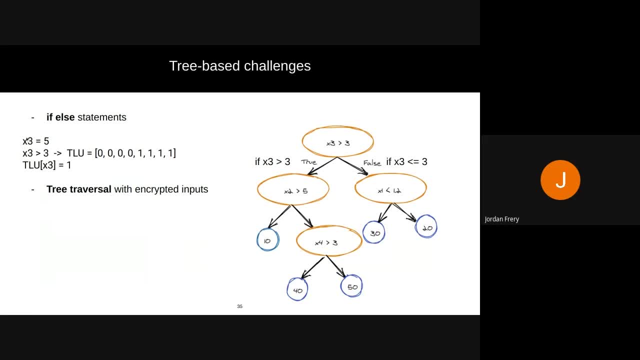 greater than is not directly possible in fh. um right, so what we do is representing this comparison with a table lookup. so imagine you have x3 here, which is equal to five. so the comparison x3 greater than three could be represented with a table lookup with only those zeros, four zeros and 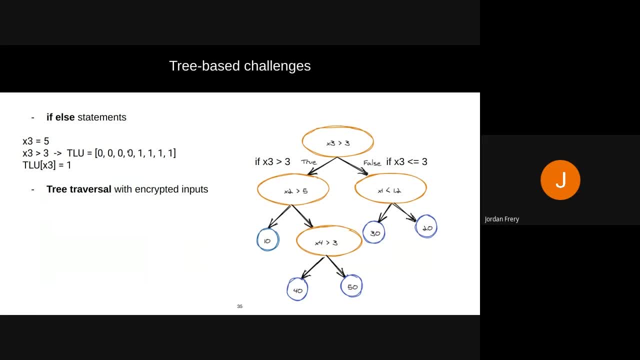 four ones. uh, what it means is that, like, look here, x3. you would just pass the x3 as the index and it will return whether it is actually, uh, greater than three or not. so this is essentially how we can do comparison in fh now. so the second part is tree traversal. tree traversal: assume that the example is only 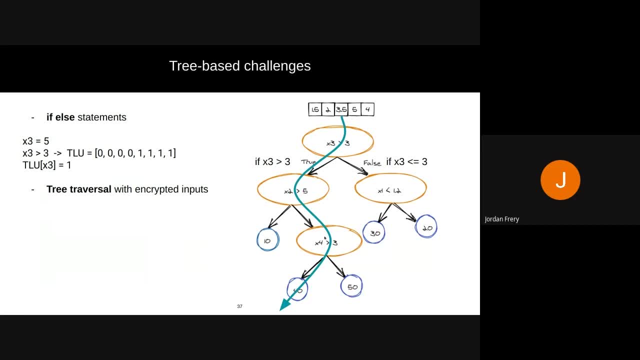 going to go through the nodes uh, that size and this is just a very simple use case in the system. so this is just a very simple use case in the system, so we have to use this to satisfy the condition. well, this in fhe is not directly. 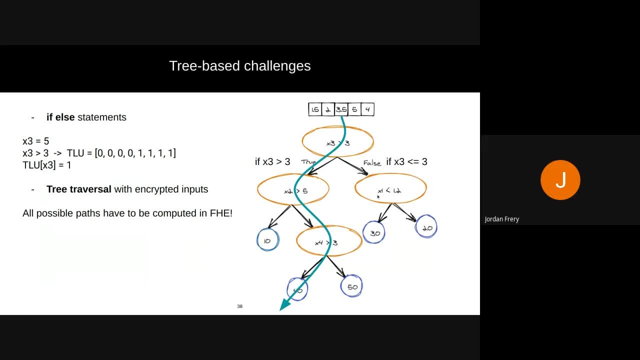 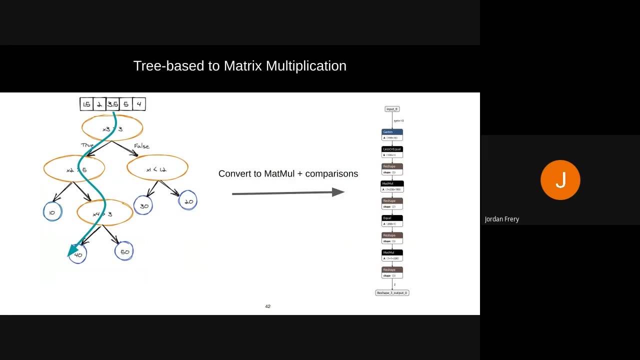 possible because fhe, like in fhe the, the input is encrypted. you can't really know. uh, the server can't really know whether it has to execute the left node or the right node. so we have to execute by basically converting the tree traversal model, like inference, to only matrix multiplications. 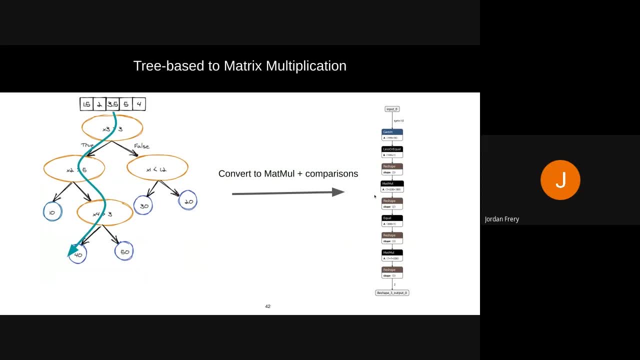 and comparison, which we can do in FHE. So with an ONNX graph it would be represented like this: A single straight graph of computations that computes every single comparison and every single condition in the tree. So this works fine for also a lot of different trees. 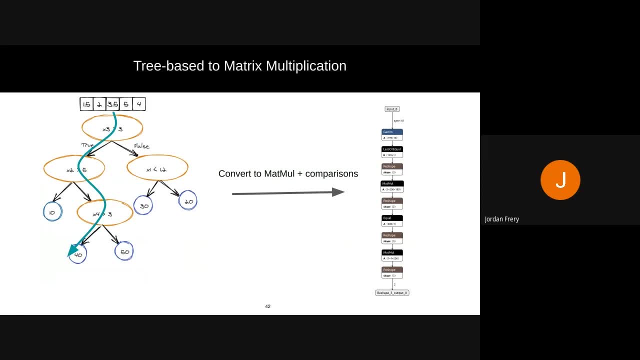 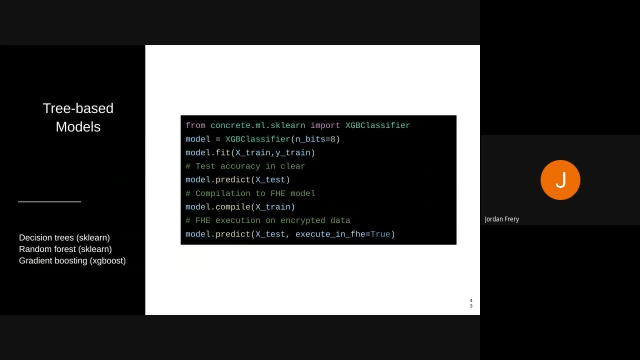 as they are in, like random forest, for example, or gradient boosting, as it basically just adds a one dimension to the matrix multiplications. Great, And- There's a question on the previous slide. Oh yeah, sorry, sorry For these trees. 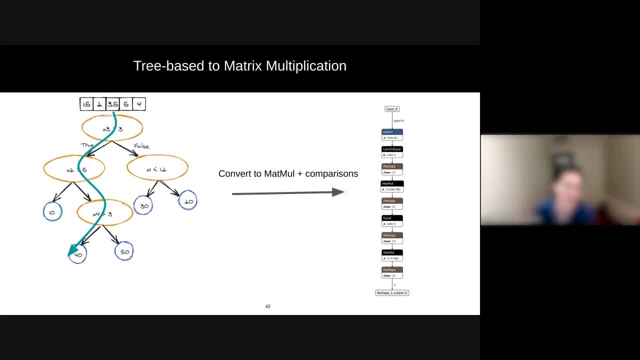 these tree-based models- and I think this question applies to a lot of other models- Was there any alternative of like converting the so like? the problem with these trees is if they're very deep, but if you're doing like random forest or something. 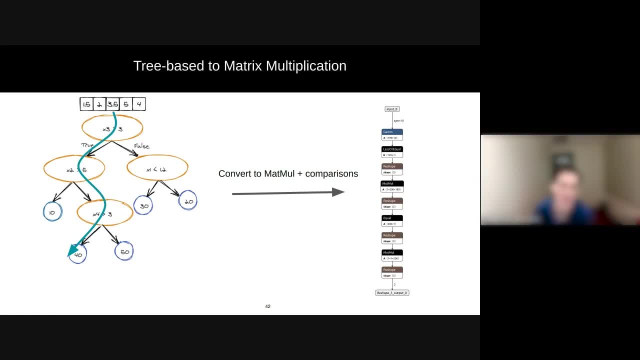 you have shallow trees, you can sort of take advantage of parallelism. Was there an attempt to like rewrite these trees in a different form that makes them more suitable for the limitations of FHE? Yeah, that's a good question. Like random forest, for example, they are gonna. 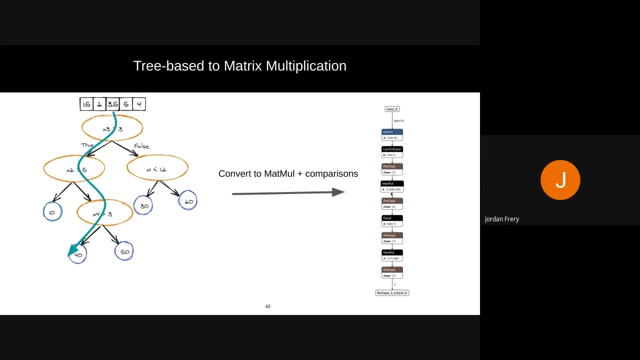 they're gonna be so deep that if you don't constrain them to stop at a specific level, then they're gonna explode in terms of matrix dimensions here. So there are. we didn't really study ways to make the random forest the entire model, with only small trees. 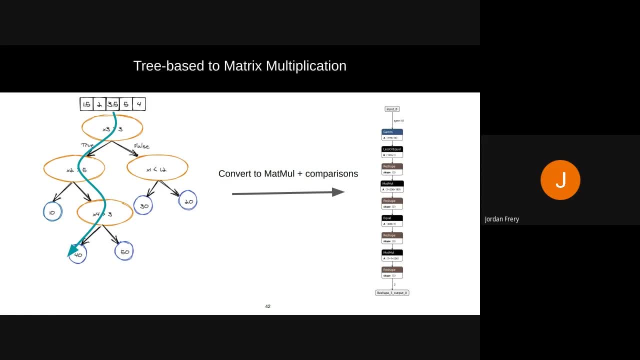 but gradient boosting, for example, is basically the inverse. You've got some shallow trees and you basically combine a lot of them, but very, very like, not deep at all. So here it's completely fine for FHE, but you're right. 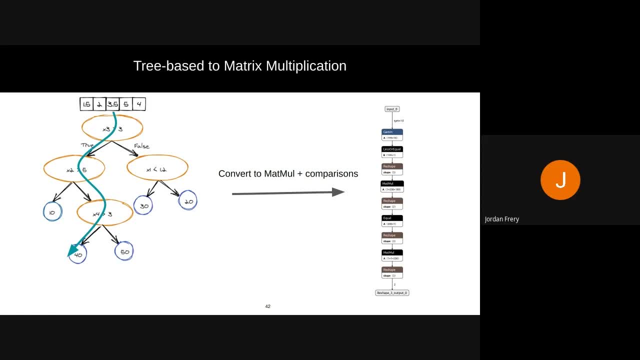 random forest in their default mode would be huge matrices here. Yeah, So I'm guessing this approach is probably taken to get all of the models into sort of the same TensorFlow graph input type of format so that they could be sort of uniform like processed, or is there like special handling? 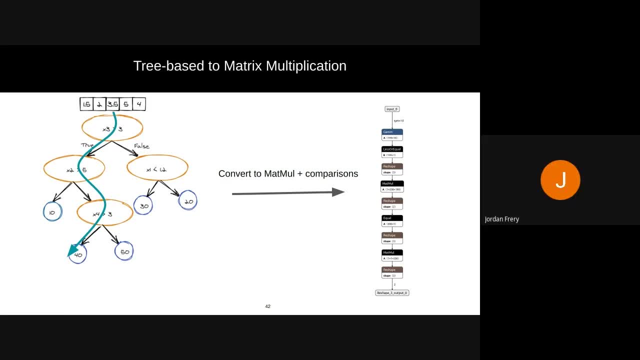 for each of the different types of models. I know. So for tree-based we use- we actually use a library developed by Microsoft called Ehrmingbird, which takes any kind of tree or ensemble of trees and transform these to the matrix multiplication representation. 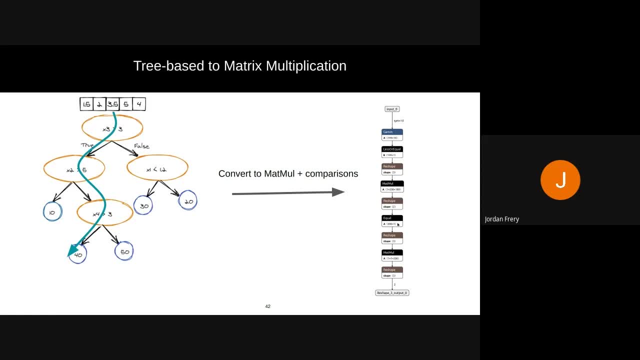 So basically any kind of tree-based algorithm in machine learning would be represented with with those nodes, Only the dimensions and the values to compare with would change. So yeah, Was that the question? Oh Yeah, thank you, Okay cool. 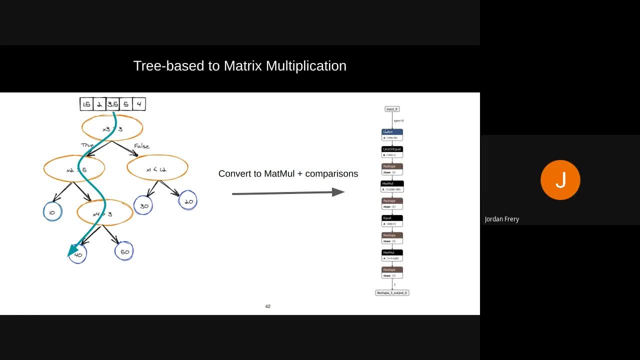 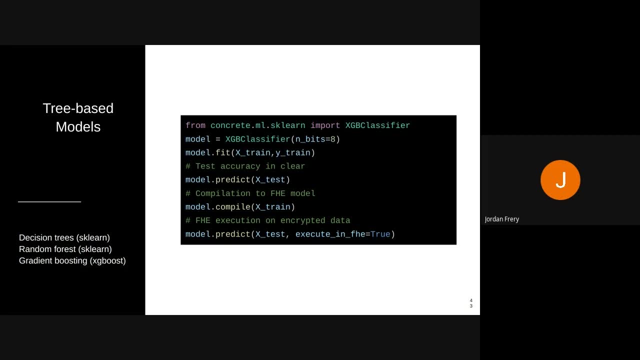 Okay, great, Okay, Okay, Yeah. So the way we use concrete ML to develop a model, to train, model and predict and stuff like that is very similar to what we would have, for example, with CKIT Learn. So you just import a model. 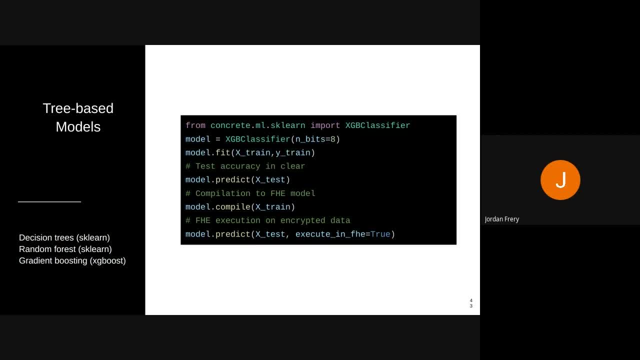 which we chose to give the same name, as they are presented in CKIT Learn or in their own library. So you just define the model And one of the most important parameter you have to give to the model when initializing is the number of bits of precision. 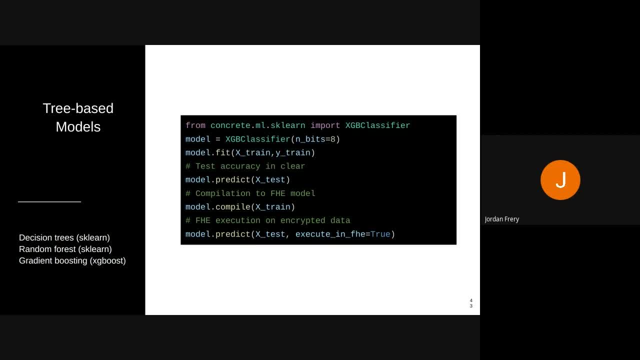 over which you want the input data to be represented. So for trees it's less constraining than for neural nets, because every single feature is going to be quantized with eight bits of precision. So you've got, for one feature, 256 different values available. 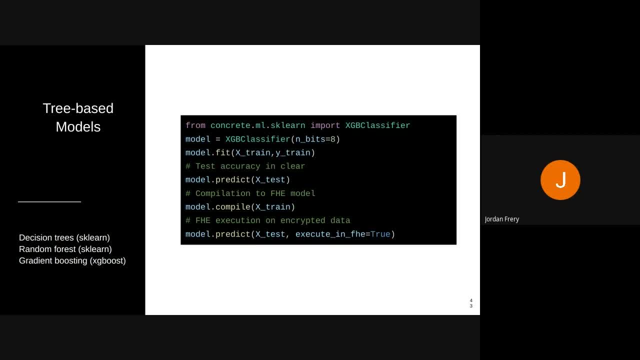 And for the second feature, 256.. While for neural nets you would have to quantize the whole input at once, because of course you send a lot of different inputs into neurons and doing different quantization, while then doing addition and quantization. 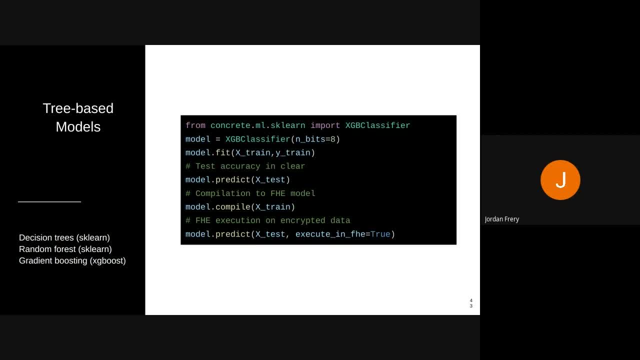 Multiplications on those differently quantized inputs would be very tricky to handle. But here, yeah, you can just train the model. So you define the N bits. you can train the model with the fit function, then call predict, which would run basic, clear inference. 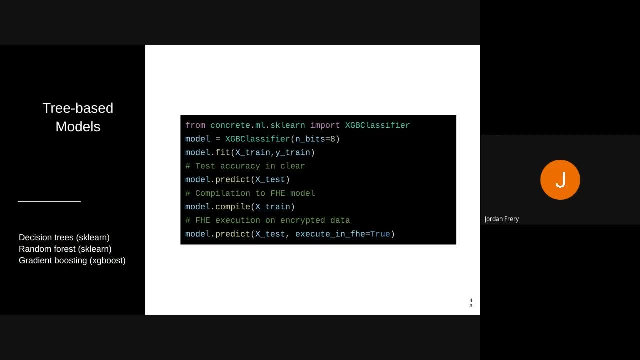 So you can actually test, debug the model, find, compute some metrics, which here would be pretty fast because it's just everything clear, But it will give you. it will give you the FHE accuracy because we run, we make sure that. 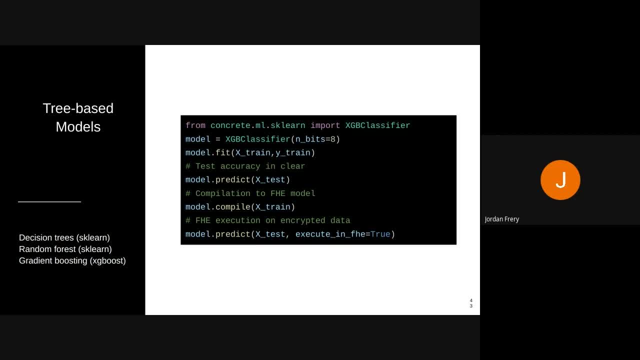 the cryptographic parameters allow you to have something like one over 100,000 chance to give the wrong output. So then you can just compile the model. This compile function is going to take some representative data sets and transform the model into different steps until it reaches the compiled 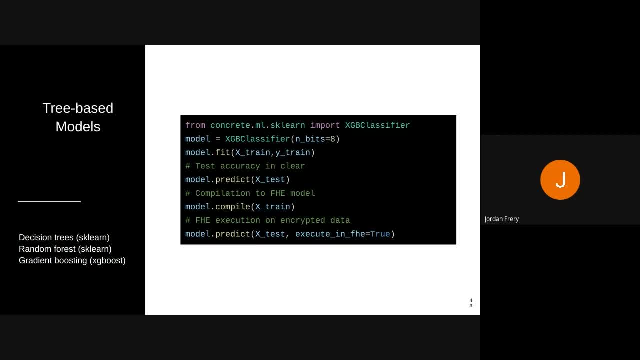 So we have an MLIR representation of the model and then we can basically execute FHE operation, pure operations, following this MLIR. And yeah, of course you can check the execution time by just simply setting the executing here. Of course, extest here is not encrypted. 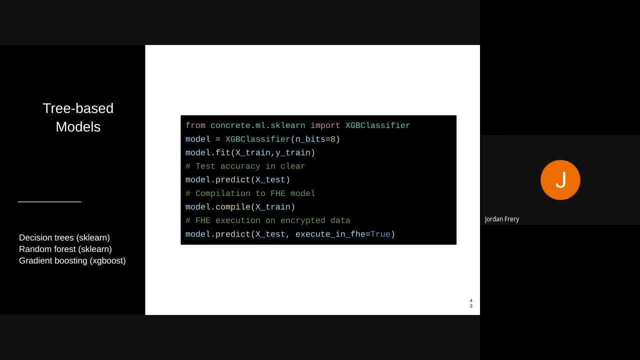 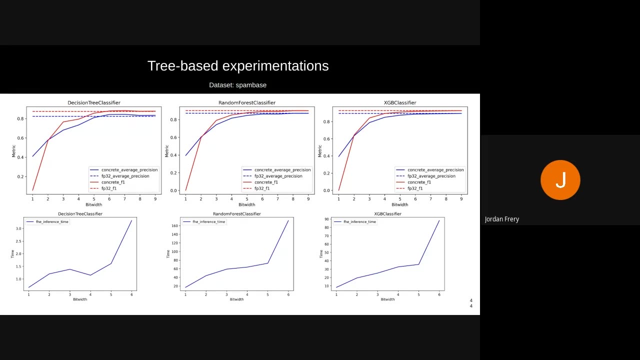 is just for debugging purposes, for data scientists, But then you can, once you are ready, you can just split the client and the server and then deploy, basically. So those are a few experiments of a spam-based dataset where we take the floating point 32 matrix. 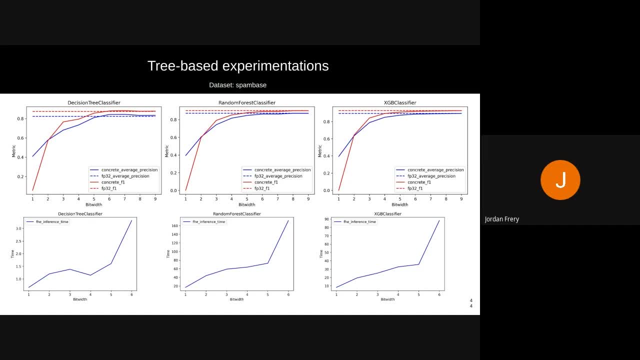 So we have the F1 metric and the average precision metric And we compute the metrics for different. so bit width would be the n bits parameter that you just saw before And, of course, with one and two year, the damage done to the accuracy. 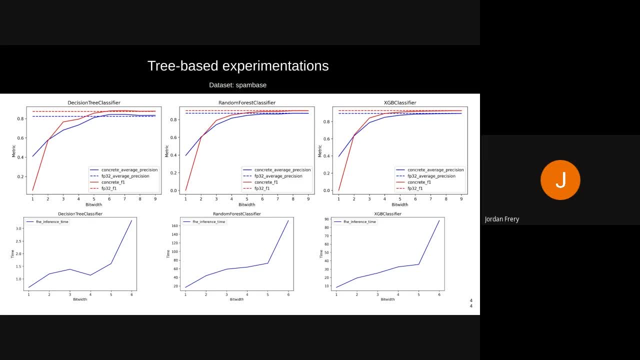 so the F1 and the average precision is pretty huge. but you convert very quickly to the floating point 32 matrix, which is great, And on the bottom you can see the inference time for all the metrics. So you can see that the F1, F2, F3, F4, F5, F6,. 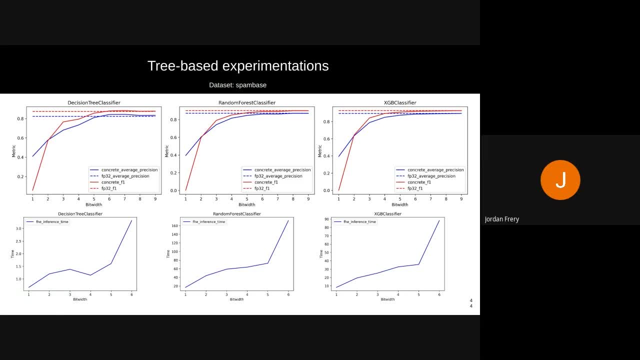 F7, F8, F9, F10, F11, F12,, F13,, F14, F15, F16, F17, F18, F19,, F20,, F21,, F22, F23, F23, F24, F25,, F26, F27, F28, F29, F30,. 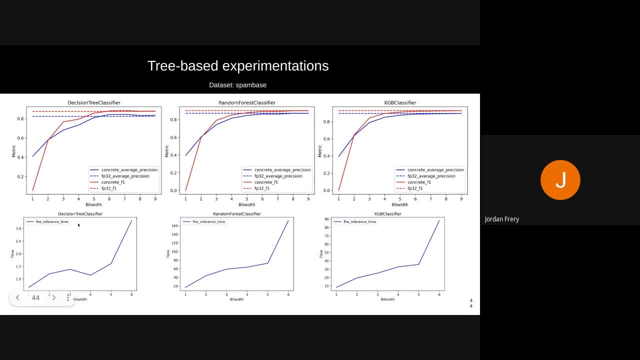 F30,, F31,, F32,, F33,, F34,, F35,, F36,, F37, F38,, F39,, F40,, F40,, F41,, F42, F43,, F44,, F45, F45,, F46,, F47,, F48,, F49,, F50,, F50,. F51,, F52,, F43,, F44, F56,, F57,, F59,, F61,, F63,, F59,, F62,, F54,, F65,, F60,, F65,, F60,, F71, F62,. 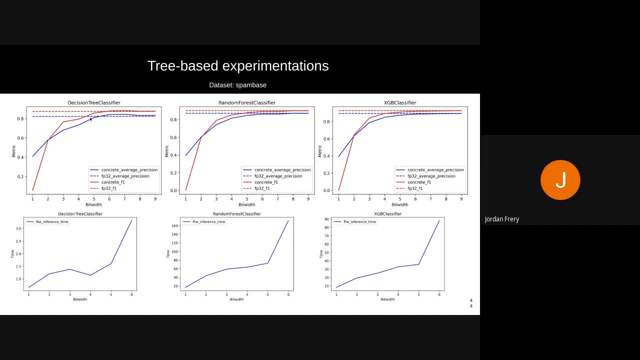 %, %, %, %, 0, %, %, %, %, %, % %. that from one to six it will triple. in terms of execution time, Random forest, as you guessed, is the most costly of the tree-based model, because it just builds very deep trees. 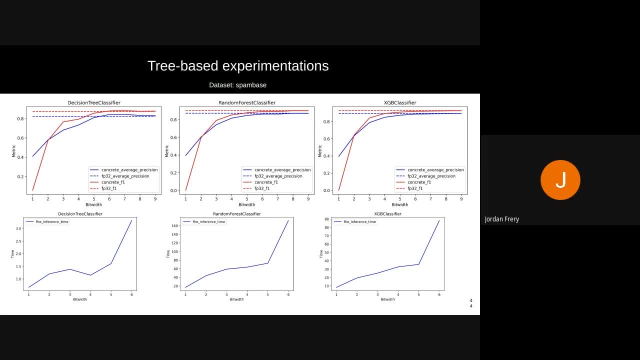 And XGBoost has a. I guess it's more friendly to FHE because it builds very shallow trees while having good accuracy. Did you say how big the decision tree classifier example was for like three seconds, like roughly? how big was the resulting network? 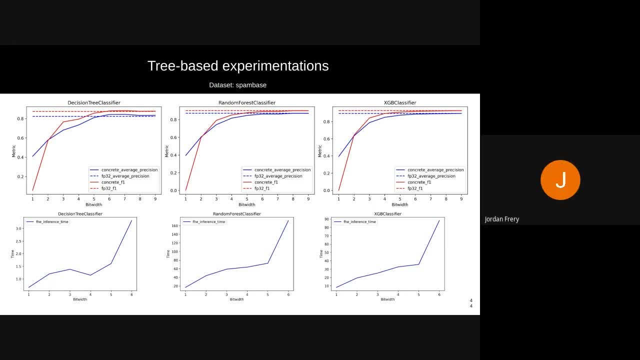 or the tree that started it. Yeah, so we don't set a limit on the depth, So it will very much depend on the data set. I can't really tell you. it's a very good point. I should actually write the complexity of the models here. 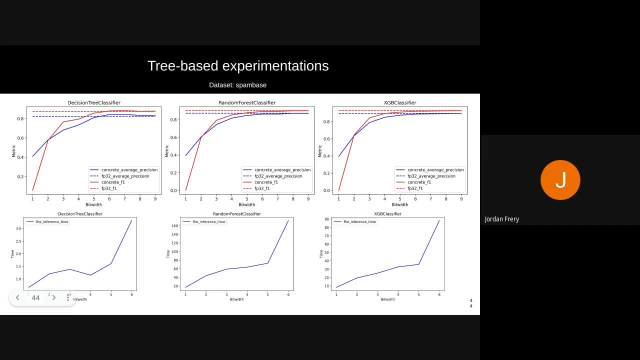 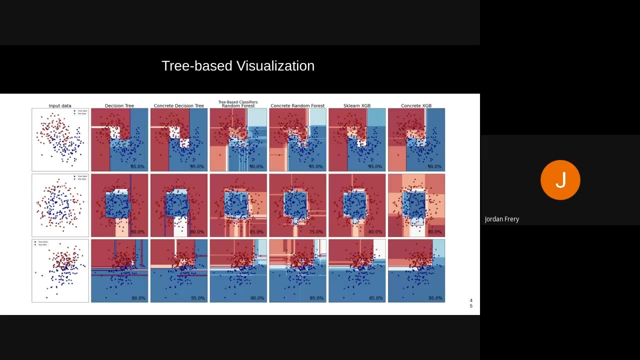 But, yeah, so it's basically trying to classify the spam-based training sets properly, But it's a single tree, while we have a hundred here and a hundred here. So, yeah, So, and there are a few visualization graphs just to show that, even though the decision boundaries, 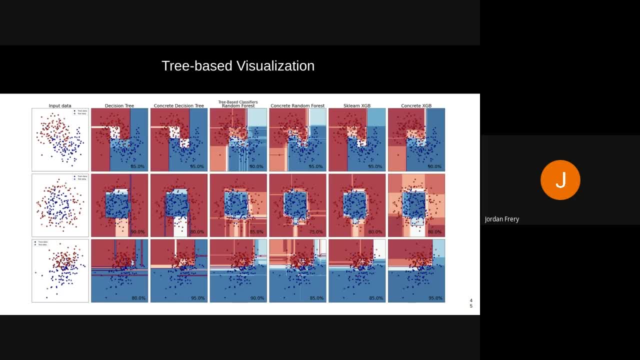 are not set at the same place because of course we quantize the input space. I will also basically quantize the output space entries Also in your nets. So you have got some different kind of decision boundaries, but the results are very similar in the end. 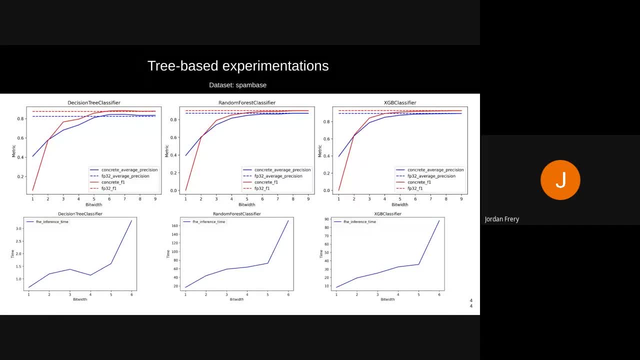 Oh, and something I didn't mention before, but we see some kind of an effect that we didn't really expect before, Like when running, that is, that quantization has some kind of regularization effects here, right, Like the concrete, has some kind of a better accuracy. 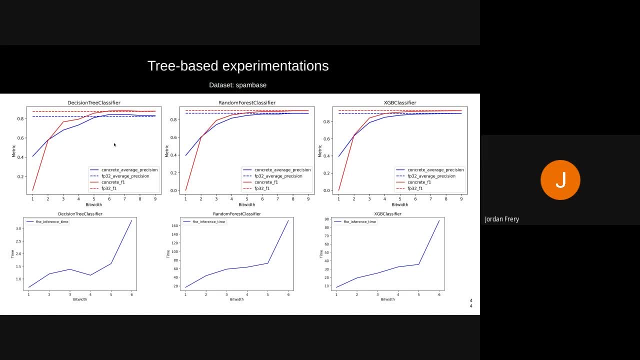 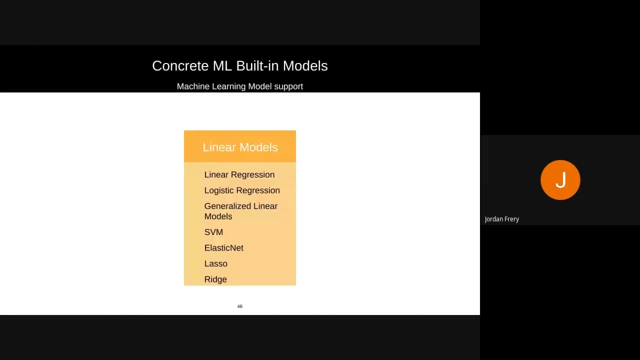 for a moment, just because quantization makes data less precise. So, yeah, Great. So now linear models. So we have a few of them. We basically tried to cover all the linear models that were implemented in SecretLearn. The good part of this is that it's very easy to use. 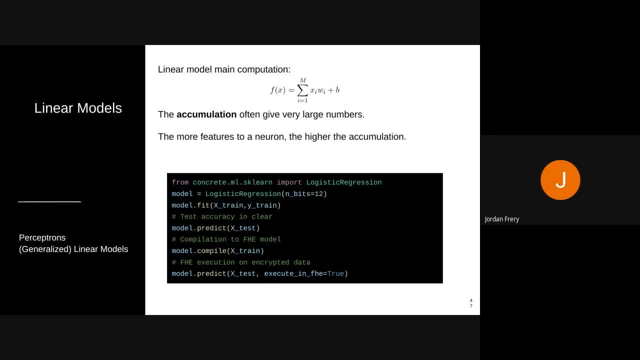 It's very easy to use. It's very easy to use. The good part here is that it is what we call leveled FHE. It's a circuit, an FHE circuit, which does not contain programmable bootstrapping. What this allows us is that we have a condition. 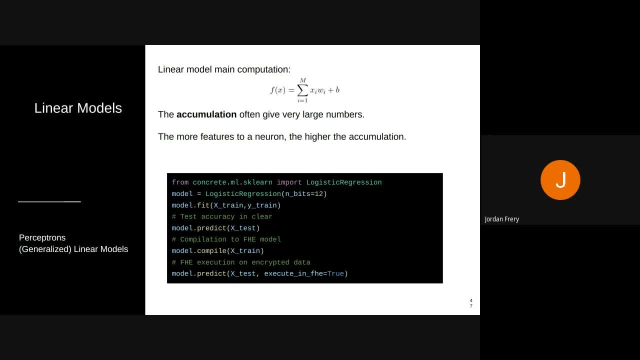 on programmable bootstrapping. that I didn't say before is that we cannot go over a certain number of bits of precision. So I can give you an example: like a year ago we were at around six bits for the input of a PBS. 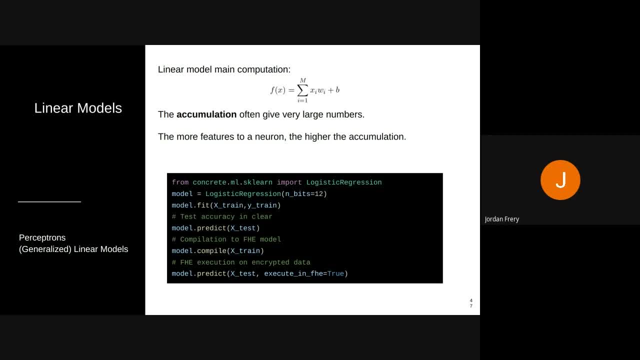 It couldn't go over that. We went to seven, eight very quickly, and now we add 16.. So the accumulator cannot go to 32 bits, but we've got like a 16 bits, which is quite good. But this does not apply to linear models. 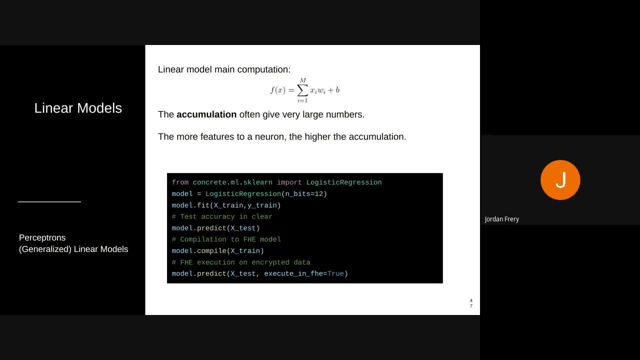 because there is no PBS. So here you can do very large sum. We can go over 32 bits, go up to 30 bits. so for example, here the number of bits we have is a quantization on the input but also on the weights. so you're going to do like 12 bits. 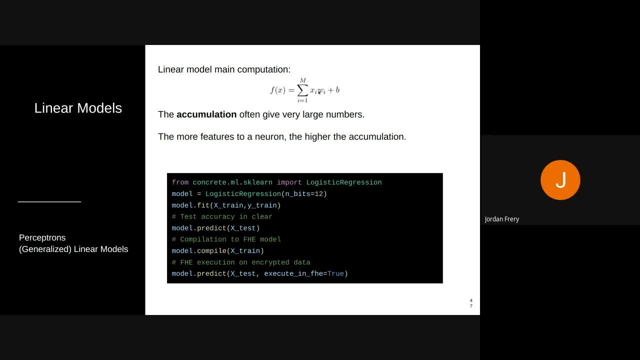 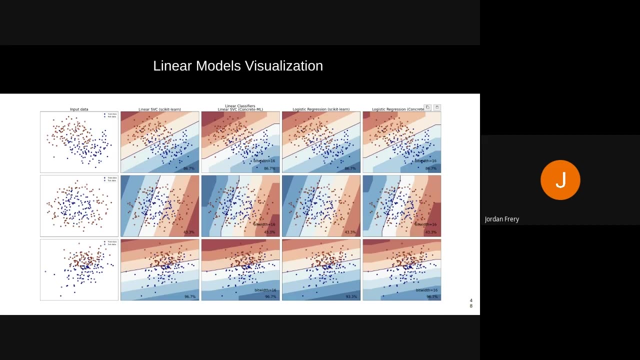 12 bits times 12 of the bits and then adding a bit bias, so you're gonna have some really large precision- uh, really large, relatively really large precision in the accumulator here. so essentially this allows us to match um the floating point 32, um accuracy, but also the run time. is is just uh. 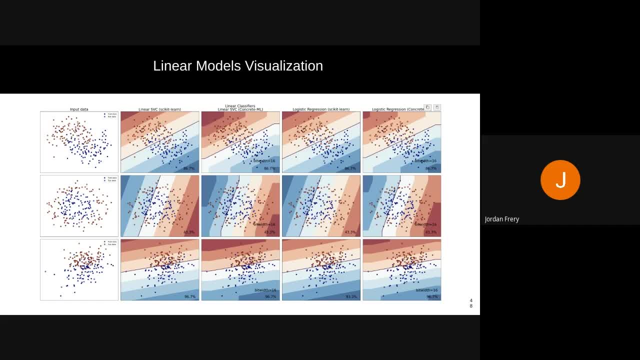 super fast. we just match uh um by it, by another of my radio, of course. uh, the floating point 32 execution time. uh, in this visualization we can see that, uh, while we are in the input range, the model behave quite similarly as the the one on floating point 32. 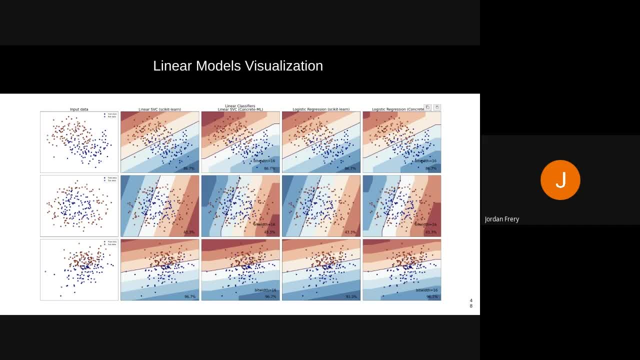 you can maybe see, like the artifact, like the, the fact that basically the quantization makes the out of bound, like out of range input, that is just without any value. so in the fhe it's uh, it's basically uh, going to overflow and this is not. 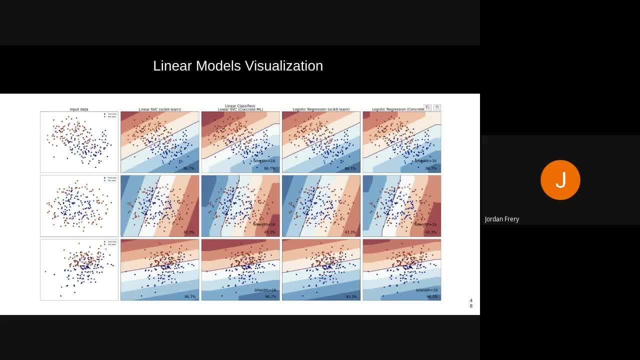 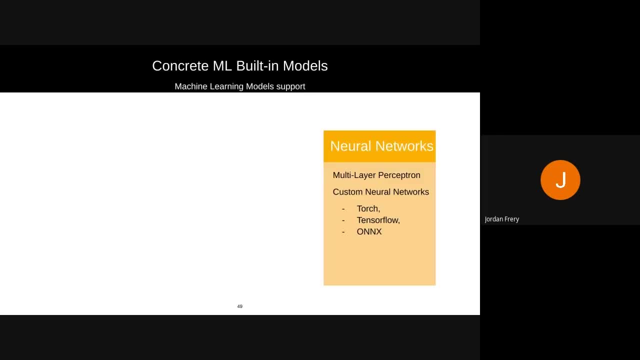 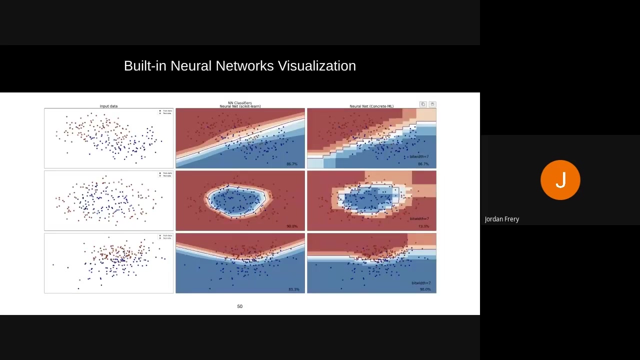 what you want. that's why, when you compile a model, you would want to give an as a representative input data point, like as possible. and now comes the last part. so neural networks, uh, the first thing is that we have built-in neural network, so essentially just a neural net classifier, neural net regressor, right, um, you can. 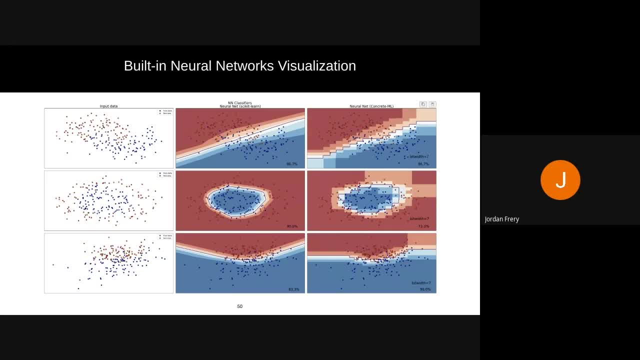 see it gives things like that. um, one complexity with neural nets is that they do very large multi-sum and then there is a pbs. so it's not like linear models. we can just have very large, uh, precision. we have to make this the accumulator, so for every single neuron you are in the neural net. 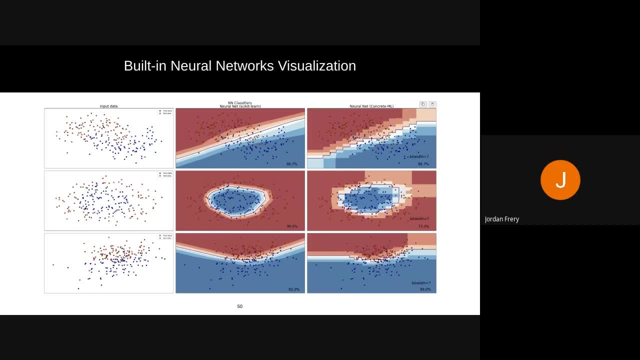 you have to uh make the accumulator uh less than 16 bits. so you can do this by either um quantizing the inputs over lower bits, or you can apply different kind of regularization to make the accumulator remain around zero. uh, there are a lot of different ways where you can also basically 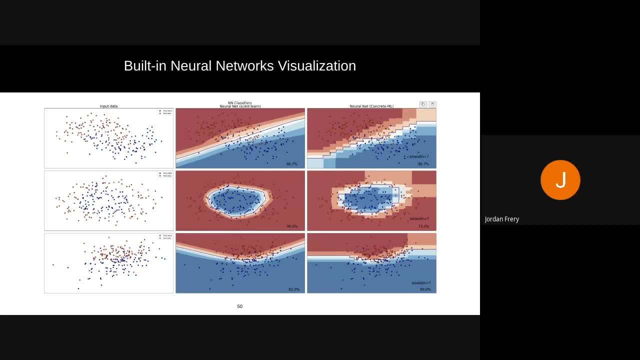 just break the matrix multiplication into several uh different matrix multiplications. but yeah, the main point is that the accumulator must not go over 16 bits to be able to use it in a pbs. so here you can see the quantization, uh boundaries, which are much less smoother. 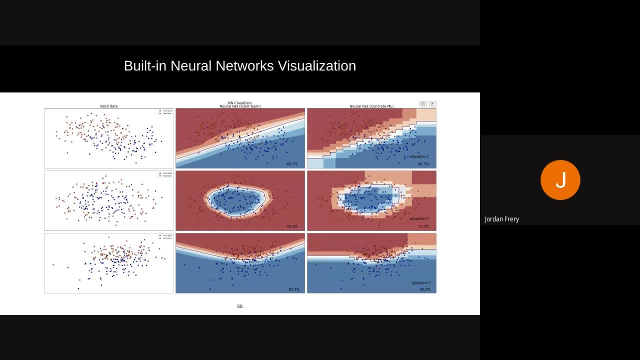 smooth, uh, smooth, that, and then the floating point, of course, but the, the, the, the accuracy remains, remains, uh, stable, um, here, to train the neural nets and make it like quantizes we are, we have kind of two different ways. the first way is training a neural net network and just 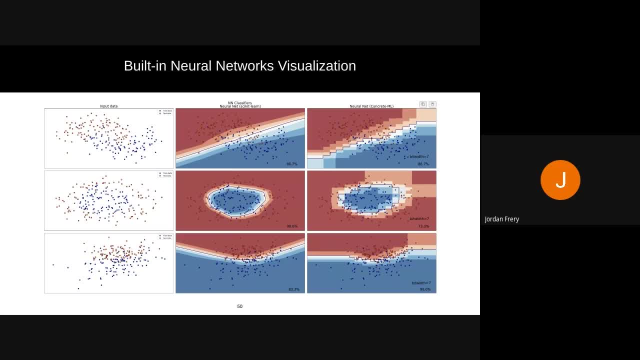 applying what we call post-training quantization. um, in this kind of quantization, you just naively: take the input, quantize it, take the weights, quantize it and that's it. you don't do anything else to your neural net. of course you would calibrate the activations. 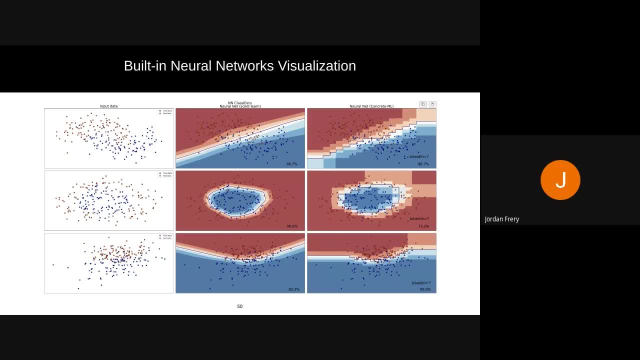 but once it's done it's done. so here, to have a bit more accuracy, we use quantization aware training, where during the training of the neural net you fake quantization. So in the inference part you apply quantization to the weights and to the activations, also the inputs. 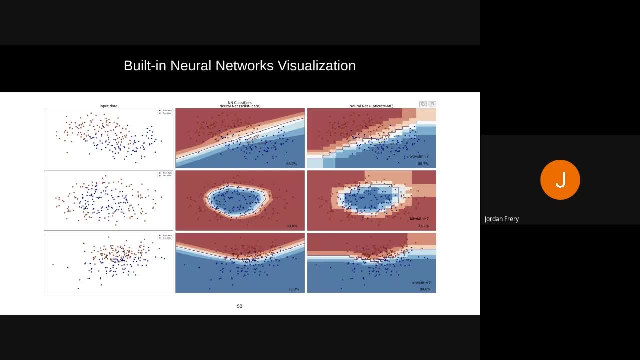 And so the neural net sees only n bits of precision. And then you apply the gradients over the 14.42 weights of course, And that way you can converge to a much better solution, which make the final neural net great. with a great accuracy we found the integers. 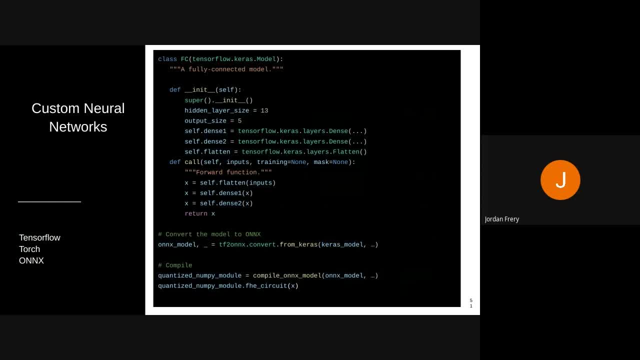 The second part is one that we are actively developing. This one is developing a custom neural network So you could take, for example, TensorFlow and create, like for example here, a fully connected model So you can do whatever you want in the model. 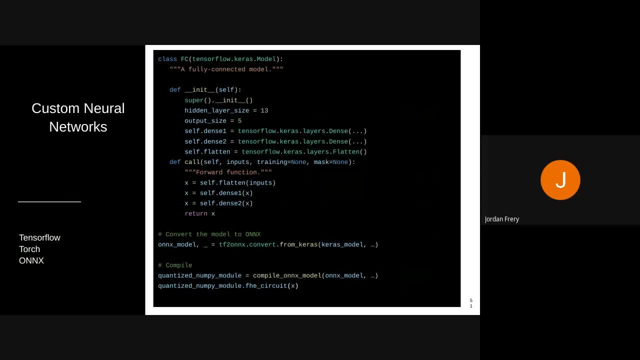 with the exception of a few operations that will be available soon but very costly in FHE. Those are, for example, ranking or doing something like max pooling, which are, you know, very costly operations. Could be done, but a bit more costly. 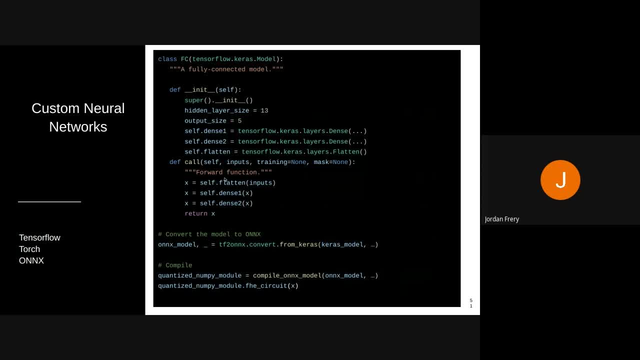 And so the first step is so: you basically create your Keras model- Let's say it's fully connected here. You transform it to ONNX- So there are different libraries that actually do this very easily- And then you can just send this into a concrete ML function. 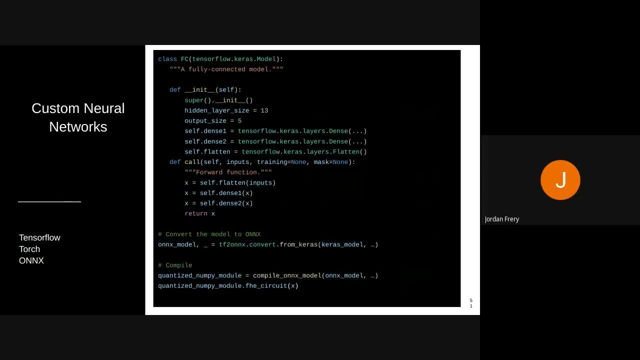 which is called compile ONNX model. So here we take the graph, we transform it to NumPy functions, and then we use another OpenSUSE library developed by Xamarin, which is called concrete NumPy, which essentially convert any NumPy functions to their homomorphic equivalent. 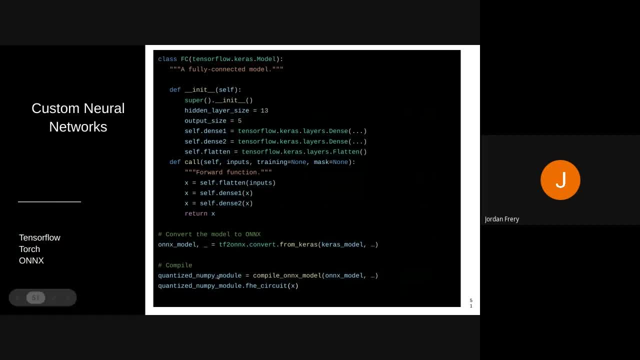 And then you can simply, so you have a quantized module here returned by a concrete ML, and then you can call this FHE circuit That can run over encrypted data, And of course here from there you can also split server client and deploy easily. 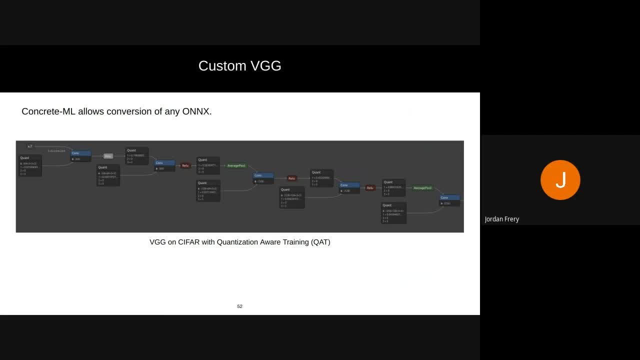 So we recently developed this for a VGG-like network using quantization-aware training. So if I plot this into a graph representation using the ONNX format, you'd see that in the graph you have some quantization node appearing. that will be very useful. 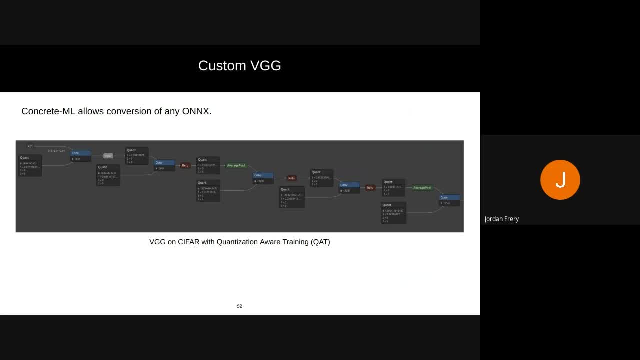 for us, because we're gonna take the parameters of this quantization and simply apply them such that the weights and the results at every output of quant node will be integers. So in the end, what happens is that the output of the convolution can be, so, must be, remain. 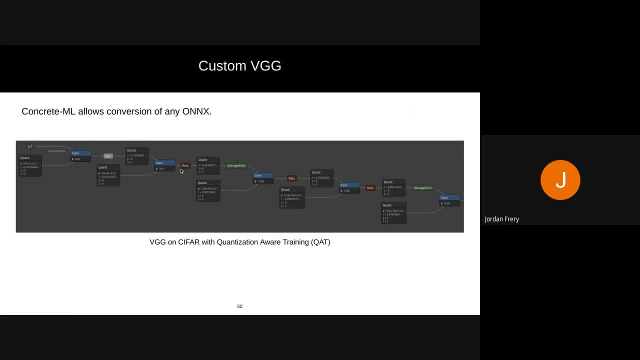 less than 16 bits. And then we make the relu, the quant node and the average, pooling a single PBS, a single PBS for every output of the convolution, of course, but we fuse them together. So, basically, PBS takes the output of the call. 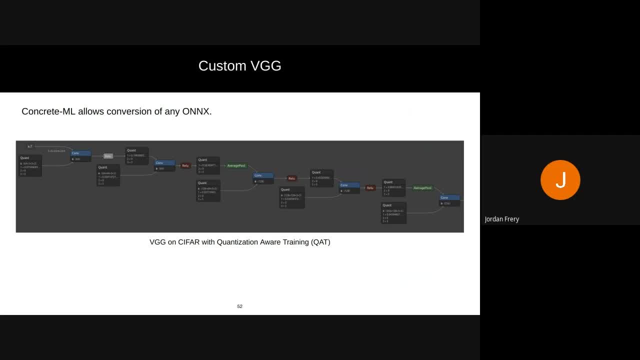 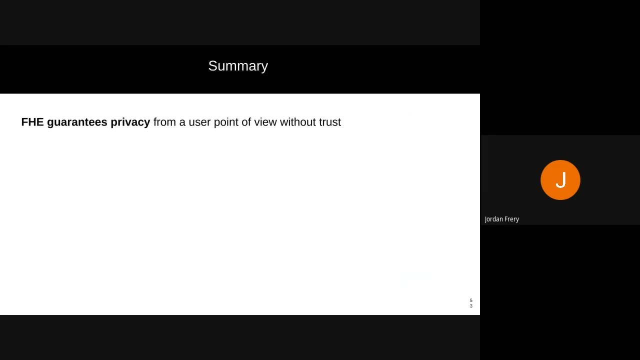 And then the output of the public of the PBS is going into the another coalition, and so on until the end of the network where the output can be decrypted by the user. Great. So FHE guarantees privacy from a user point of view. 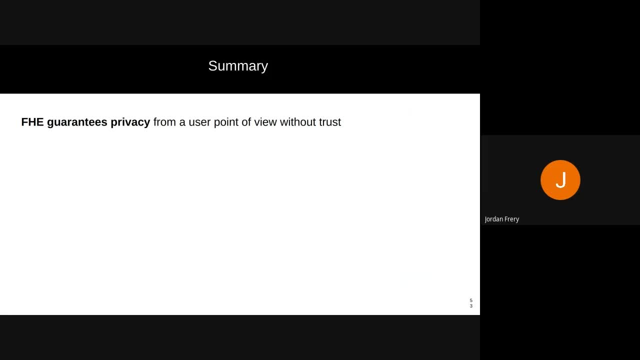 The main thing here, I think, is to remove trust from the process of the user asking a service to a third party, Because trust is not needed. The server is actually just selling a service and the user wants the service. The user just shouldn't have to trust the server that it's not going to leak the data. 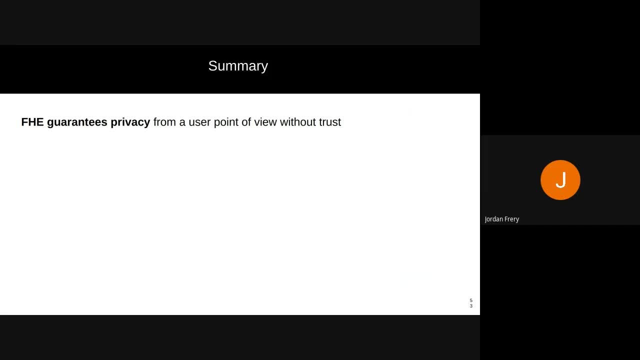 or whatever. Actually, even for the server, it has an advantage because data leak out, Yeah, So that's one of the things that we see happening very often, even though it's not actually the will of the company. Quantization is a heavy part of our open source library, which is a necessary step to convert. 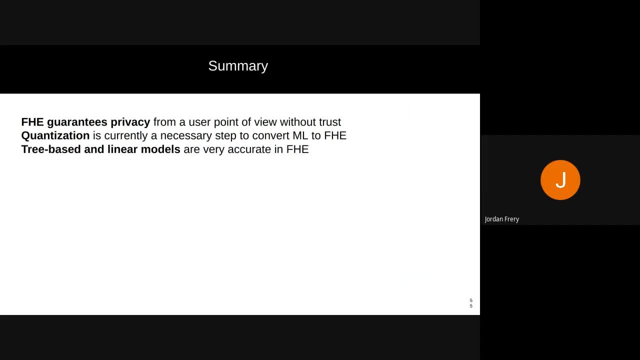 machine learning model to the FHE equivalent. We have tree-based model and linear models which are very accurate in FHE. So, of course, if you take a random forest and you have a tree, you can actually convert the tree to a machine learning model. 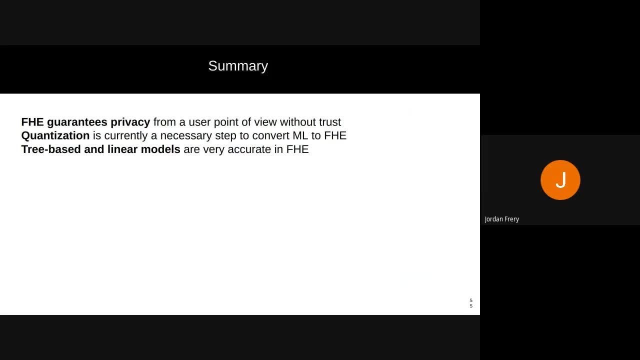 So that's one of the things that we're trying to do. Great. So the next thing is to try to have the largest random forest. You're going to have some trouble, But, for example models, they perform really well with shallow trees. 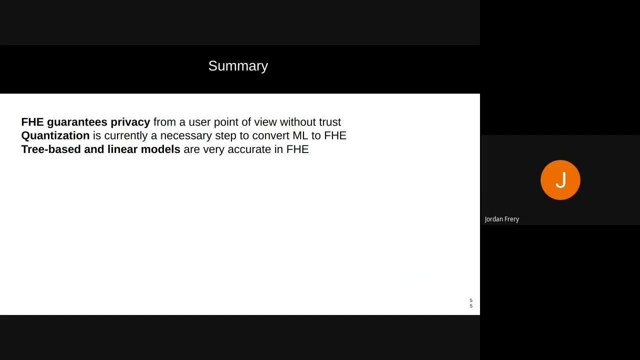 and give some very accurate results. And linear models are just very, very close to their F floating point 32. equivalent Neural network can be more constrained. These all come from the fact that the accumulator even in quantization real. in the research it's very often assumed that accumulator are not quantized. so even though 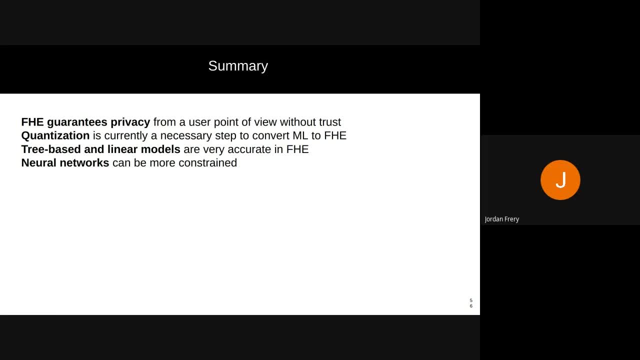 they quantize, even with low bits, inputs and weights. they just don't quantize the accumulator. so they have a 30- 32 floating point accumulator that is freely available, like other parts also mentioned that the input, for example the first layer of a neural net, shouldn't be quantized. so